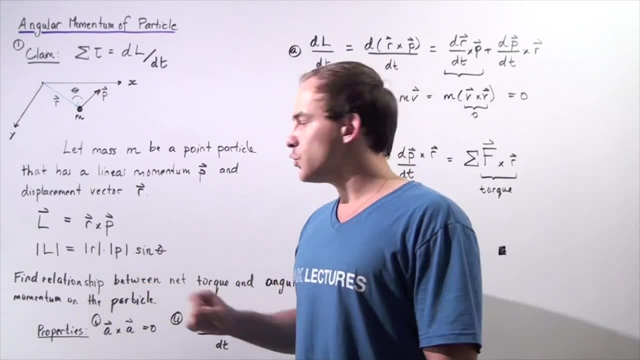 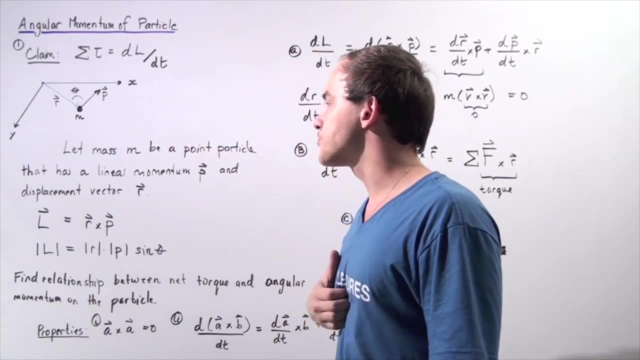 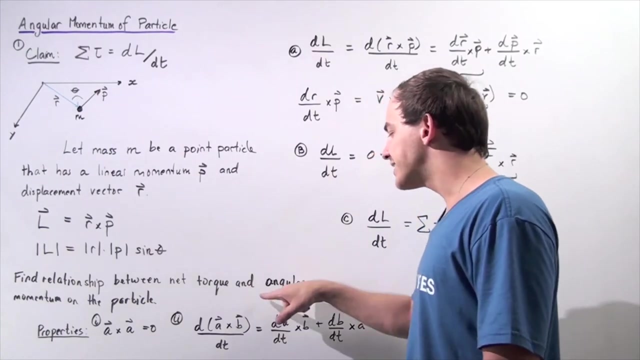 of the magnitude of the r vector and the magnitude of the p vector and multiply by the sine of the angle theta between our two vectors. Now we want to actually find the relationship between the net torque acting on our object and the angular momentum of our point particle. 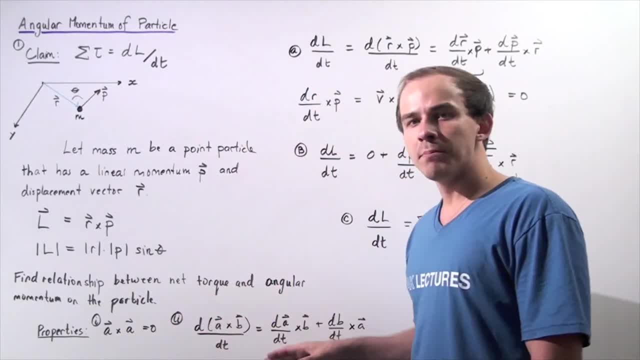 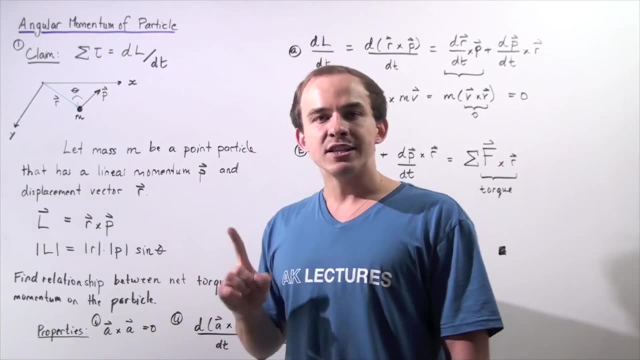 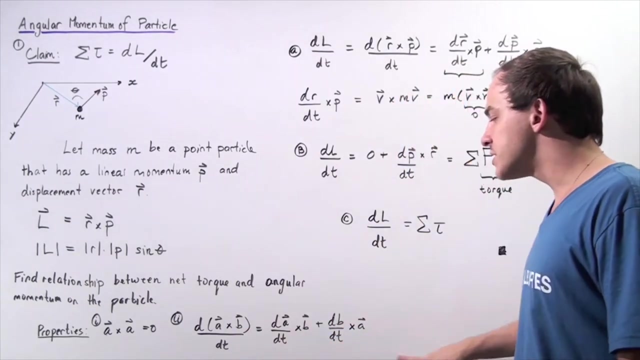 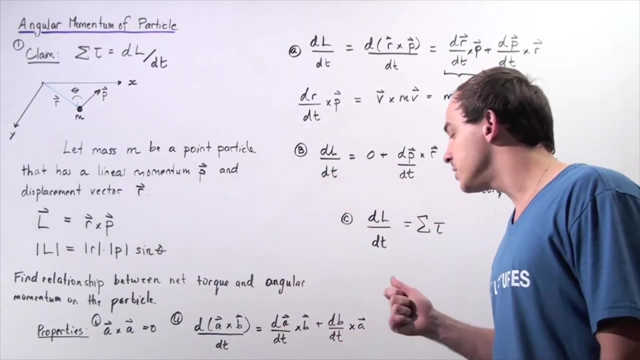 So before we begin, let's review the following properties of cross product. So if we have a vector a and we have a vector b and we take the derivative of the cross product of vector a and b, we get the following results: This is equivalent to the derivative of our vector a cross vector b. 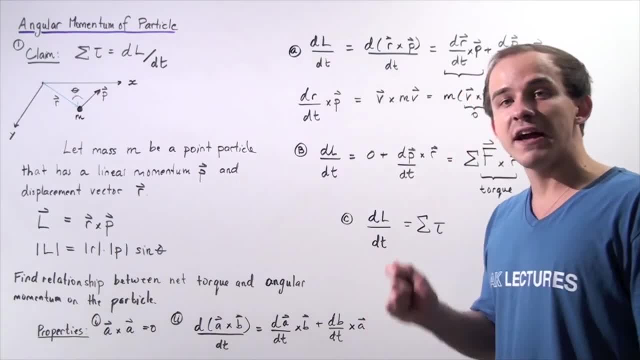 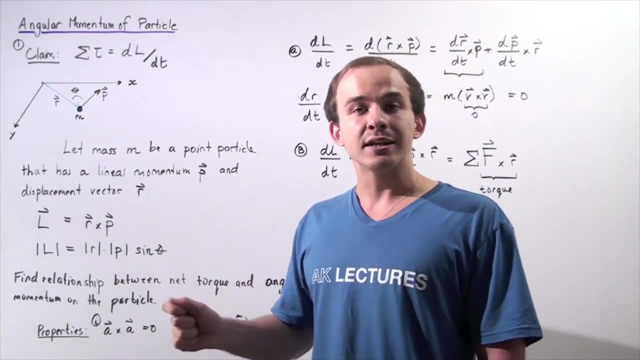 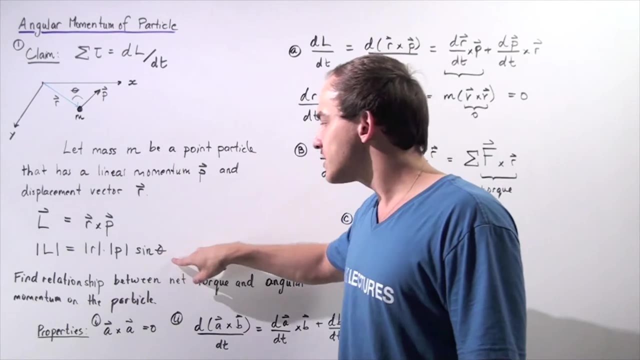 plus the derivative of the vector b cross vector a. And if we take the vector a or the vector b and take the cross product of itself, for example a cross a, that will give a zero. And that makes sense because the magnitude of this quantity sine of the angle zero is zero. 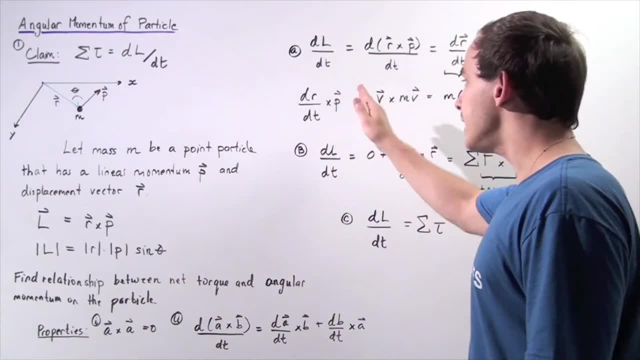 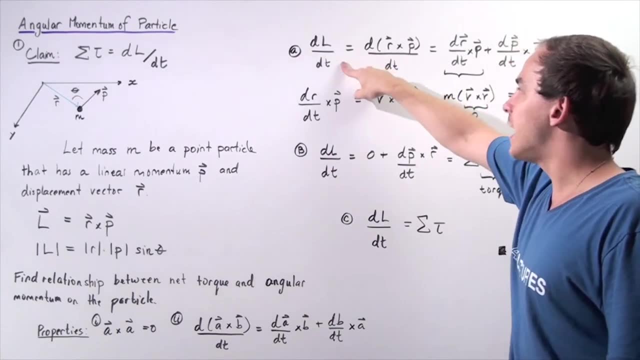 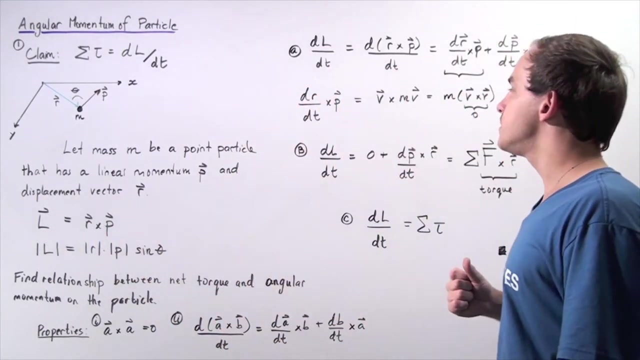 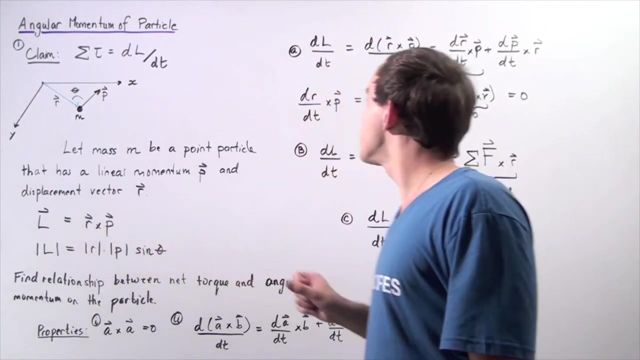 So the entire term becomes zero. Now let's actually show that this equation is actually true, And let's begin with the following relationship: So we take this equation and take the derivative of both sides with respect to time. So dl divided by dt is equal to d cross product, r cross p. 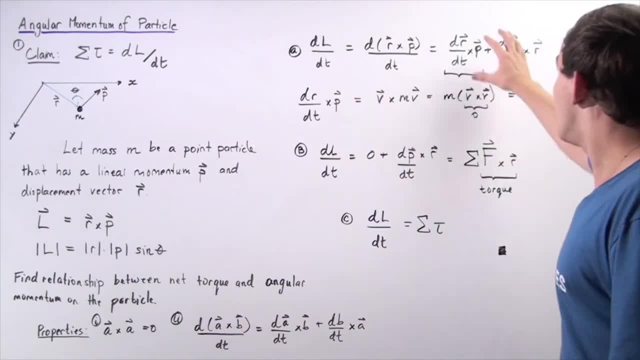 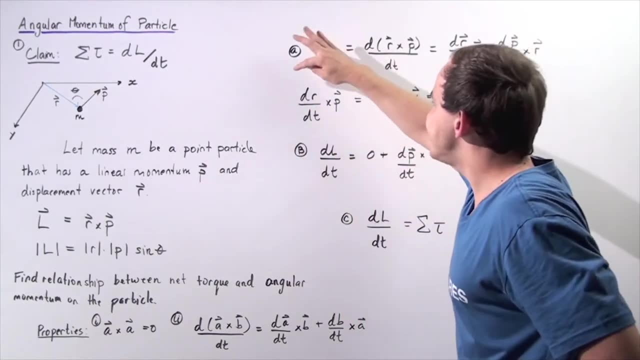 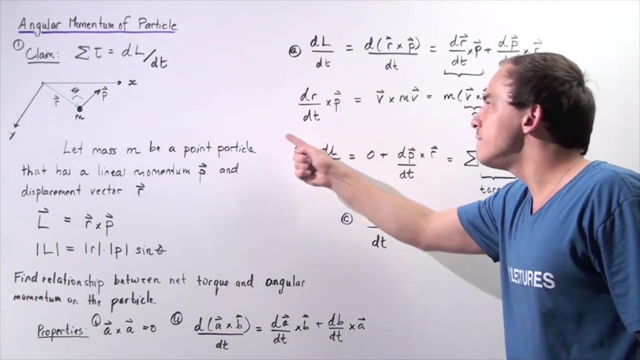 So notice, now we use property number two and we get the following result: So now we take the first term and we place it here And notice that dr, with respect to time, Is equal to the velocity. In other words, the derivative of our displacement function with respect to time is simply equivalent to velocity. 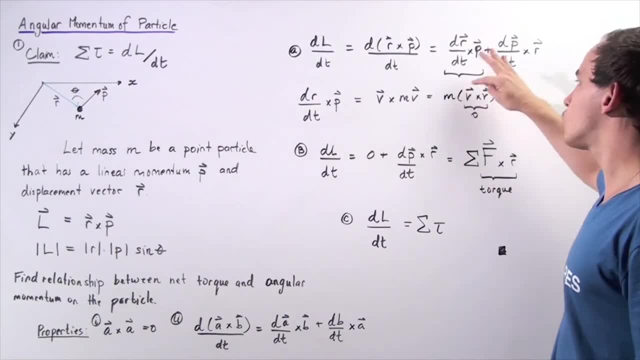 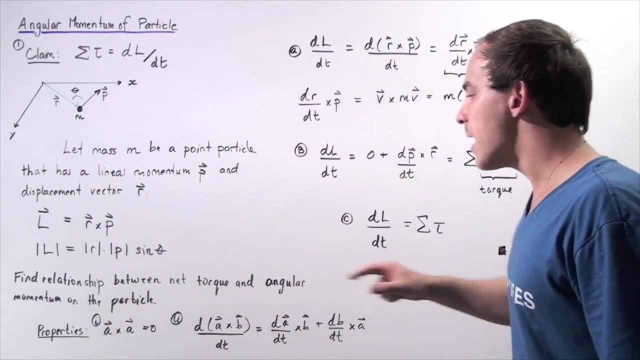 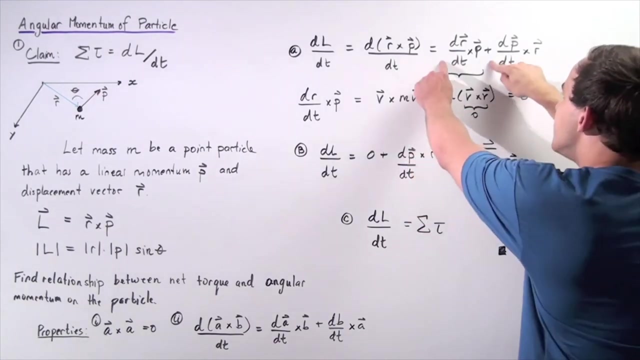 And v cross mv is the same thing as saying v cross v multiplied by the scalar quantity m. Now notice, according to property one, property i, v cross v is simply zero. So that means m times zero is zero, And this entire term.